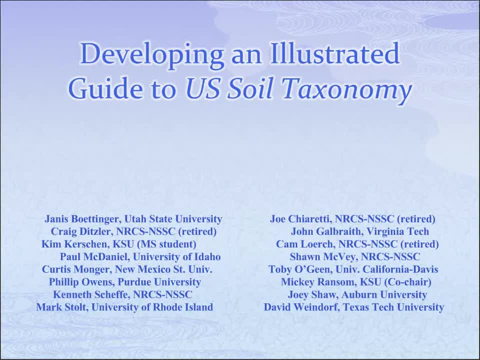 a situation where it was becoming more and more difficult to teach US soil taxonomy. One of the things- I guess Sean's put up the first slide now- is talking about the developing of an illustrated guide to US soil taxonomy. It's been quite a collaborative. 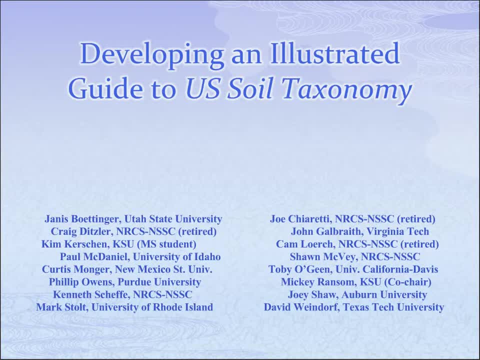 effort that went into this. You notice there's about 16 names listed there, About half NRCS and about the other half- maybe a little bit more than half in fact- are university professors and or professors, And about the other half are personnel. The roots of this go back to about 2011,, Asheville. 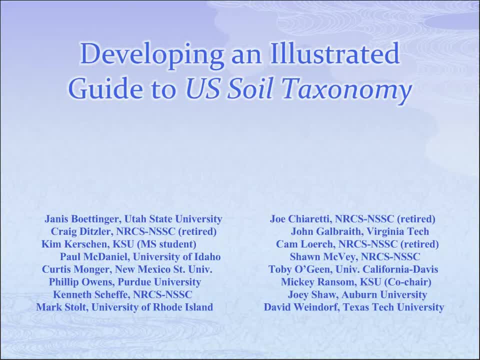 I think it was at the National Cooperative Soil Survey Conference. Casual comment by- I think it was quite probably Mickey Ransom, since he was selected as chair of the work group. A casual comment to Mike Golden: was this thing's so hard to teach you know soil? 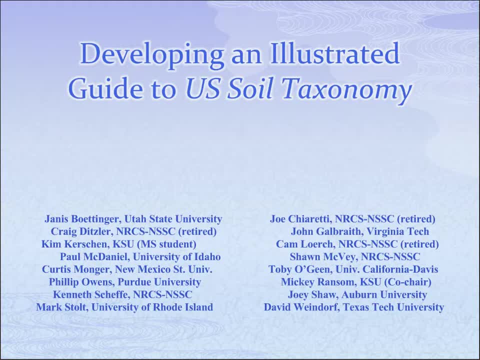 classification, And out of that came a concept and an idea that we need to do more of this, something about that, and so a work group was formed with Mickey Ransom as the chair, as well as Cam Lurch. he was a, of course, now retired, but he was the. 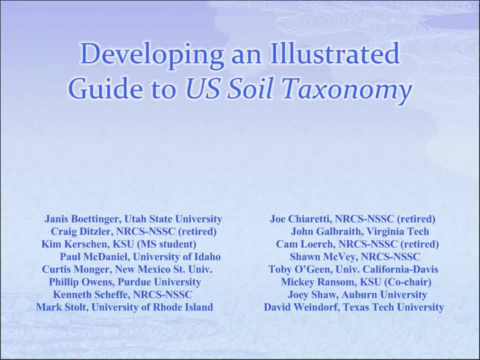 co-chair until he did did retire. others involved: Janice Bettinger, Utah State. Craig Ditzler, who's retired. he used to be our national leader for standards. Kim Kurchin- kind of an interesting thing there. Kim was a graduate student at Kansas State and her thesis was teaching of soil. taxonomy are the keys. 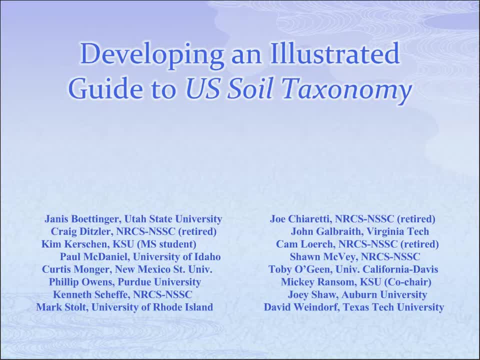 to soil taxonomy using the keys themselves and using at that time, the first product created for this was the was a simplified guide soil taxonomy, and so she made her thesis into comparative analysis of the student performance on the teaching of these methods, and she just successfully defended her thesis on. 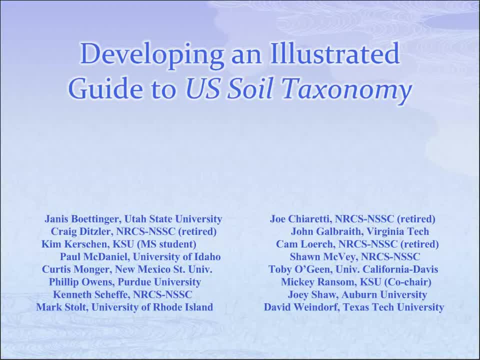 this early this past summer on that subject. others involve Paul McDaniel, Curtis Munger, Phillip Owens, Mark Stolt, Joe Sciarretti, who's retired, John Galbraith, Sean McVeigh, Toby Ogeen, Joey Shaw and Dave Weindorff at Texas Tech. 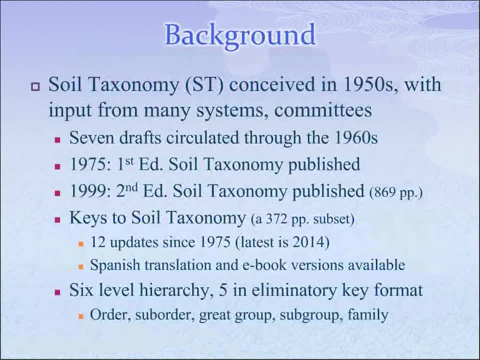 you got the slides there, Sean. a little bit of background, I think you know. many of you who have studied soil taxonomy know it was first conceived back in the 50s. we were looking for a classification system to organize our knowledge about soils. the first issue of it- we first of all, I guess, had the 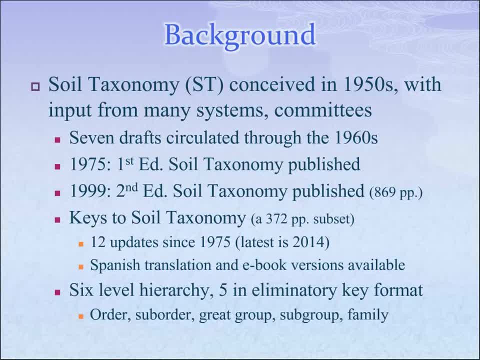 seventh approximation, issued sometime in the in the 60s, giving a begin the initial stages of what we have and know as soil taxonomy today. in 1975 the first edition was published and 1999 the second edition was published. if you remember, the first edition is about two inches thick, the second 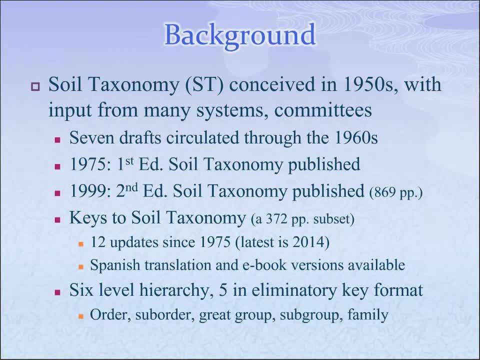 edition four inches thick, and the second edition had less photos and more taxa and criteria regarding soil classification. Mary Jo has left the conference during this whole time as interim steps were made in soil taxonomy to keep up with this and make these changes available to the users. the keys to soil taxonomy were: 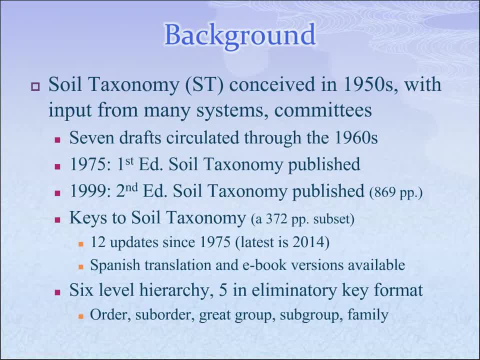 published on a basis of about once every three to four years. right now we have the latest one is our 12th edition of the keys to soil taxonomy, and it was just released this past May. we also might also add that probably in the future, look for that summer schedule and and to issue a release of the of a new 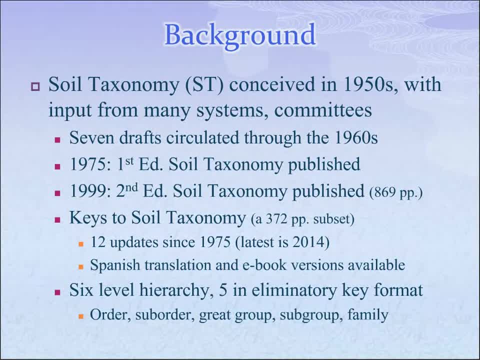 version of the keys that kind of coincides with the world congress of soils or congress of soil science. yeah, so we're going to try to stick to that once in four year rotation or sequencing. Spanish translations are available for the keys to soil taxonomy as well as it. 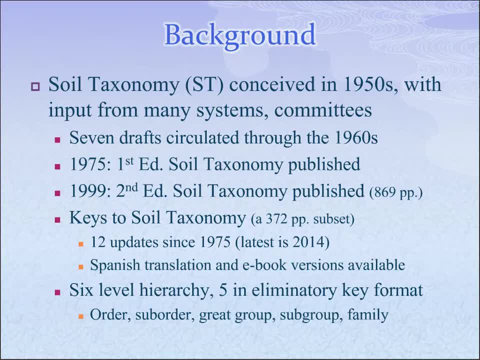 you've probably seen, it's on available on an e-book format to and electronically for your mobile devices. many probably don't know, but there are six levels of hierarchy within soil taxonomy: their first fiber and what they call eliminatory key format. that means as you move down, you step down through the 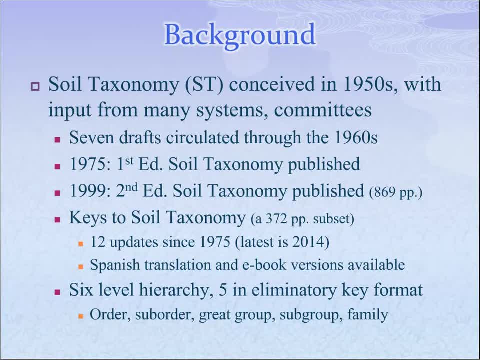 system and it takes you on a defined path to a final tax or final classification. the lowest level of that, or the sixth level in the hierarchy, is the soil series, and probably many of you have familiarity with the soul series concept, of course, and I think for full series that we have there's around 24,000 soil. 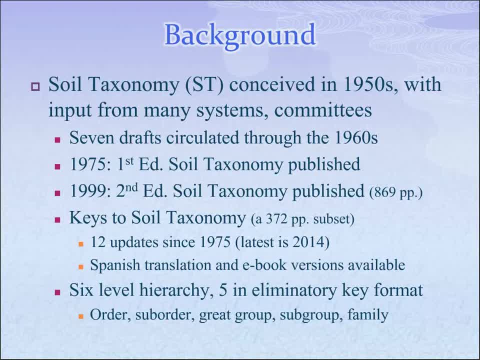 series recognized in the US, as of the last check we did, and worldwide, easily about 30,000 soil series. of course we don't keep track of all those in our soul series database that we maintain here at the center, but that's a lot of full series now and in a lot of countries you know. so taxonomy has been. 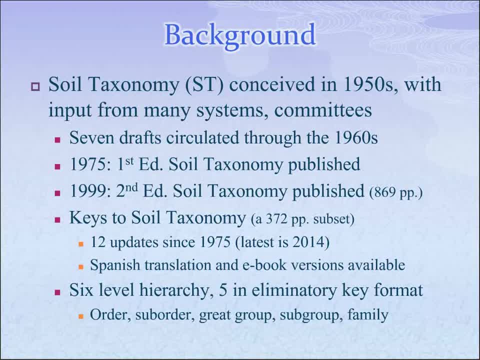 around since 75. so a lot of countries have adopted some of the concepts and some of the structure of soil taxonomy into their own classification systems and, like you know, some of you were, I was in Ireland and their classification system draws a lot upon US soil taxonomy. it's not the same, but it draws upon a. 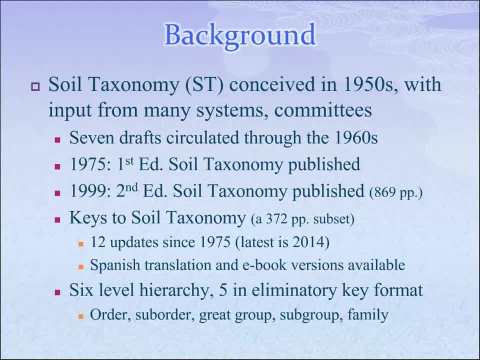 lot of concepts that were developed there, and there was a great deal of a ability to communicate and in terms of, well, how does soil tech? and we were studying the WRB or world reference based system, and they would ask: well, how does that relate to soil taxonomy? and so that was a one of the things: to kind of give you an idea. they 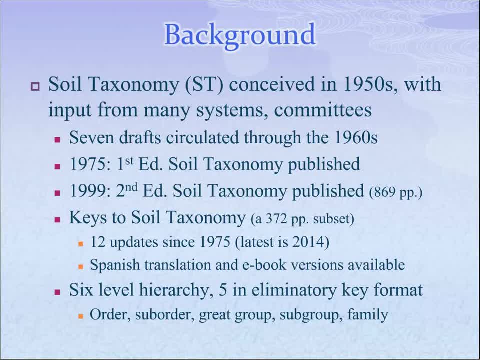 the widespread at least understanding and use utilization of soil taxonomy. come on, got it over here. so some of the strengths of the system is: every soil is allocated to a class through the FACAPs and it's classified in the FACAPs and they're classified based on the 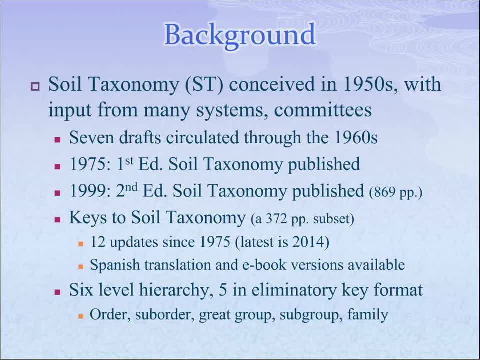 size of the system, so you're sometimes given the place to choose the soil type- family level. The system also strongly enables soil survey production and interpretation. Okay, You know one of the good things about it: you can make decisions right in the field. 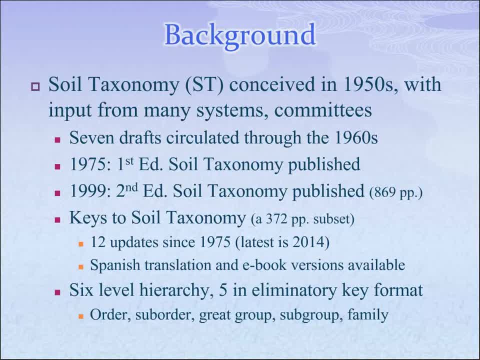 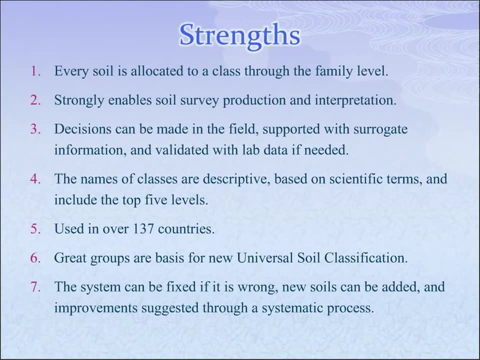 when you're using soil taxonomy, And the one thing that, of course, it does make tremendous use of is ancillary laboratory data and such The names are somewhat descriptive. The names are, you know, in terms of within the classification based upon scientific terminology, at least. 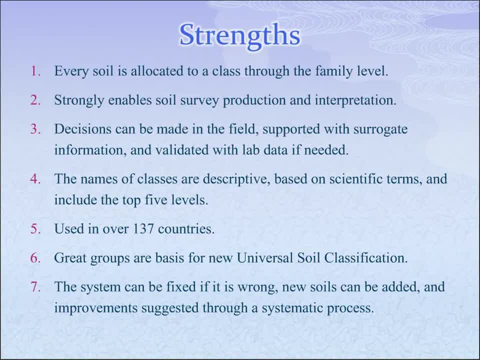 at the top five levels. Soil taxonomy, like I said, is widely used: 137 countries have utilized soil taxonomy at some point in time- And my understanding of not having been a part of this yet, but the universal soil classification system, which is being looked at and possibly developed through the International Union of Soil and 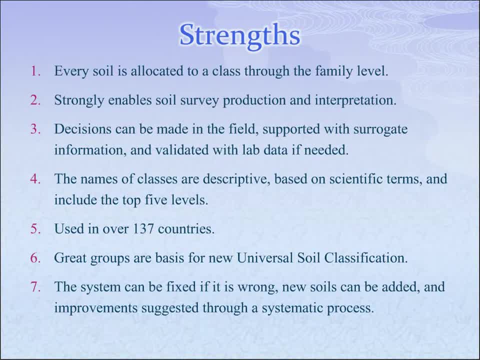 Soil Science. they are looking at our great groups being the basis of that classification system, And I just want to point out that one of the nice things about the soil taxonomy system is every soil in the world can be classified. Somehow it'll fall out through the family. 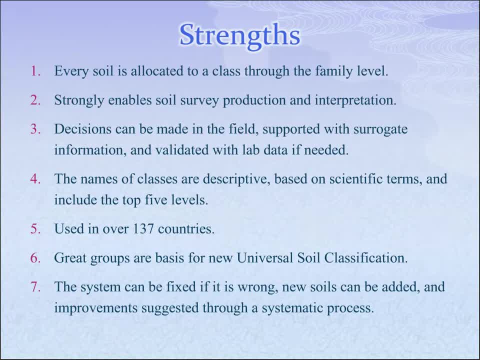 level And soil taxonomy is also a common language for comparison and research, As was mentioned. you know, if the system's wrong we can fix it. Just make a suggestion And it's improved. You know those systems are going to be more efficient And it's going. 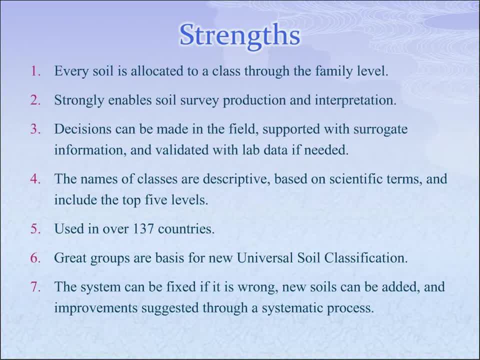 to get better and better And there are a couple more things that we have to get going on with soil from thevadorg, 168 countries have made changes, improvements like that They come through the standards branch here at the National Soil Survey Center via regional soil survey conferences, national 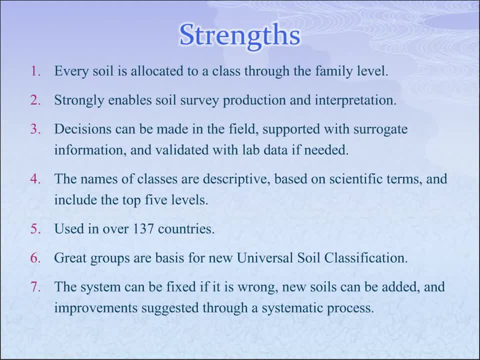 soil survey conferences, or just simply submit it to the director here and he'll get it to where it needs to go. Joel O 마스크, Yeah, we'll be submitting our publishing an update to Part 614 of the National Soil Survey Handbook here, probably within the 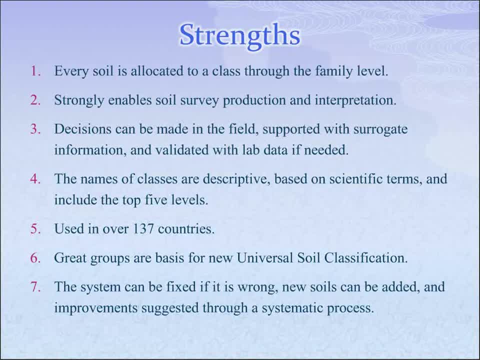 next month or so. So and that update gives a clearer picture of how the processing of amendments to soil taxonomy is going to proceed. It'll be a whole lot more open and a whole lot more transparent to those who make proposals and those who are viewing the status of the analysis of proposals to change taxonomy. 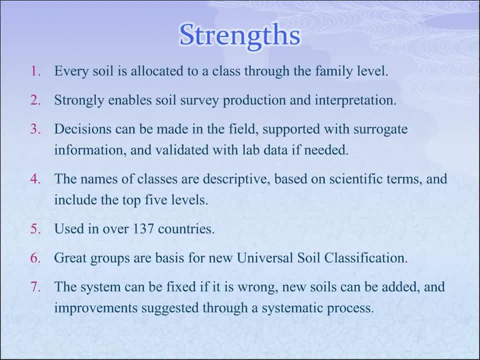 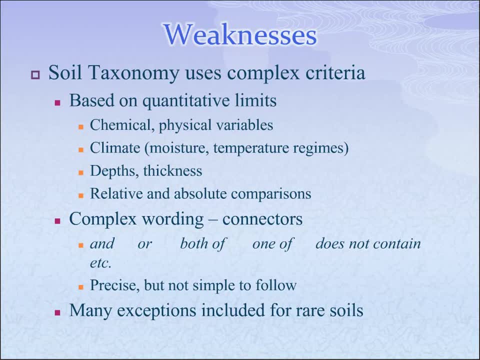 But there are some weaknesses to soil taxonomy. We'll be the first to admit that. Okay, the weaknesses are. the main one is: it is incredibly complex Those how many of you have tried to use it in the room here? Two or three, four, yeah, okay. 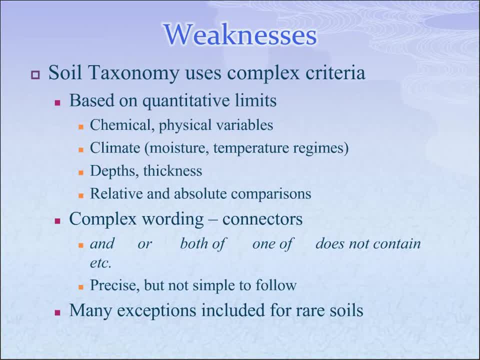 Have tried to use it and you probably do understand how complex it can be. It one of the things that makes it complex. it has quantitative limits. You know for percent base saturation, how much organic matter salinity. various of the taxoclases have numeric values. 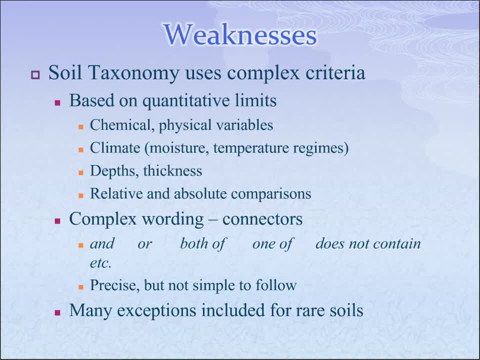 For the quantification of that factor within the soil. Not only do you have that, but it has to occur within certain depths within the soil, And so that adds additional complexity to the whole system. You have chemical and physical variables, climate variables such as moisture status. 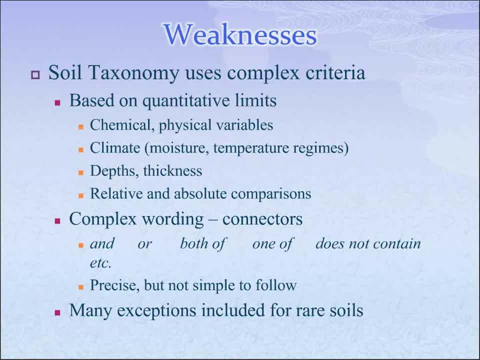 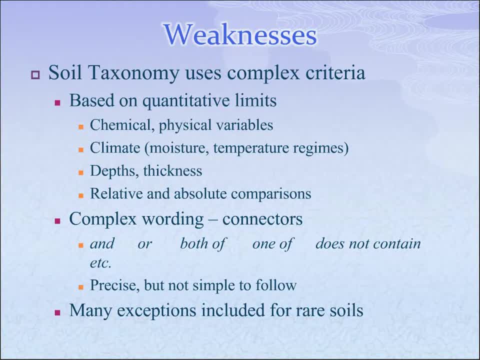 complex wording: and or both of, neither of, or and or. this that does not contain, et cetera. These are the kind of words that it uses. It makes it rather complex to visualize what you're actually classifying. 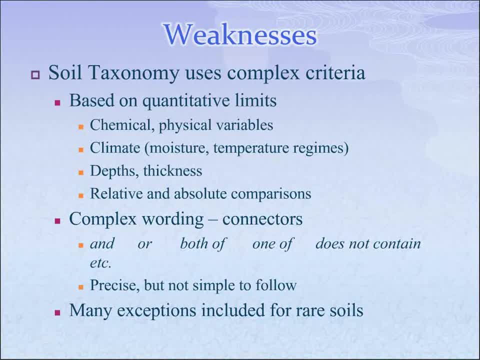 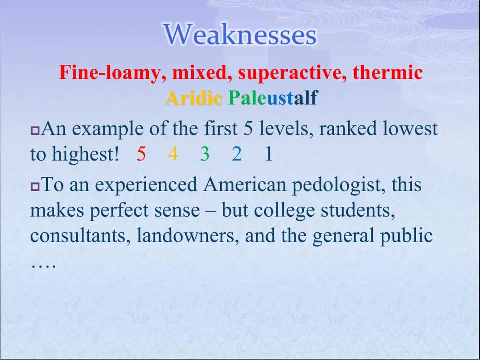 It's precise, but it's not easy to follow. There are also exceptions that are made within the taxonomic system for the for those rare soils. Some of its weakness, of course, is it's very long, rather long taxonomic class that we have there. 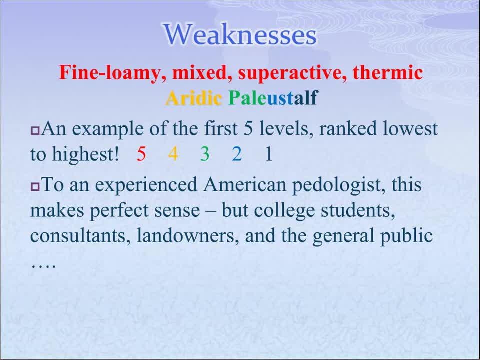 Looking at the one that you have on the screen there, fine loaming mixed superactive thermic. Now that is the terms used in the family classification level within soil taxonomy: The, the one in yellow there, eridic. that is the fourth level, which is the great green. 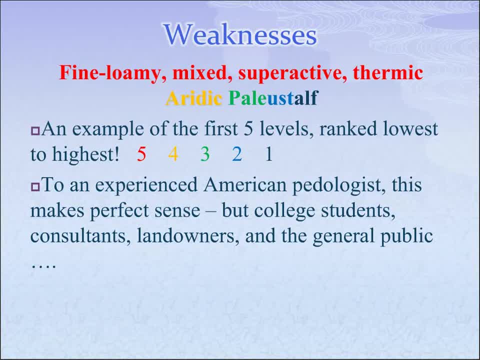 And then of course, subgroup level- I mean subgroup level, I'm sorry- And then of course three, two and one or great group suborder and order in that order. To someone experienced in using soil classification or pedologists, it makes perfect sense. 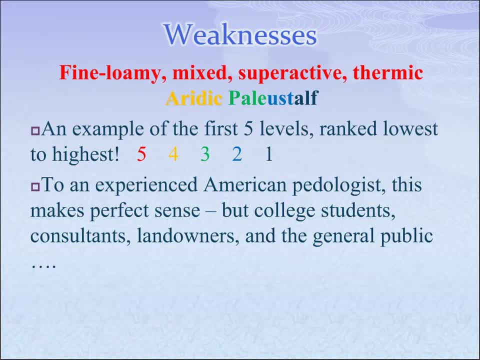 It's kind of a hierarchical structure of building from the base up upward through the soil family. But if you're not involved in soil classification, soil taxonomy, soil mapping, this is probably, you know, a little bit of a challenge. 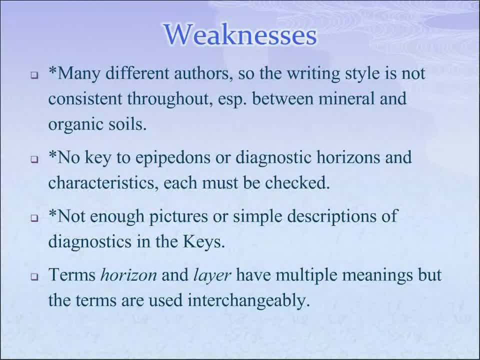 More difficult in Greek, I would say, And there's lots of different authors that come. You know, very few of us have seen soils from all over the world, all the continents, And so there's been many different authors, So the writing style is not exactly consistent throughout. 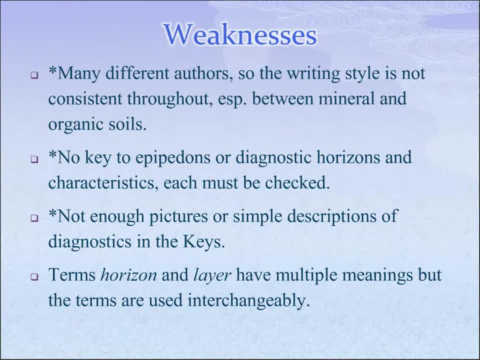 especially between the mineral and the organic soil. You know, and there's no key to the epipedons or the diagnostic horizons and characteristics. Each one has to be checked. That's the way it is now And there's not. 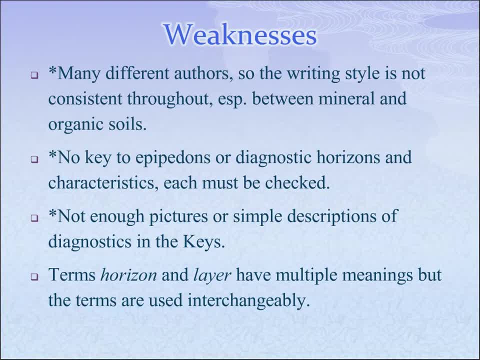 A lot of pictures in the keys or simple descriptions, You know, and also terms. horizon and layer have different meanings, but the terms are kind of used interchangeably depending on where you look in the system. Now it's interesting to note these first three that we've identified, the number of authors. 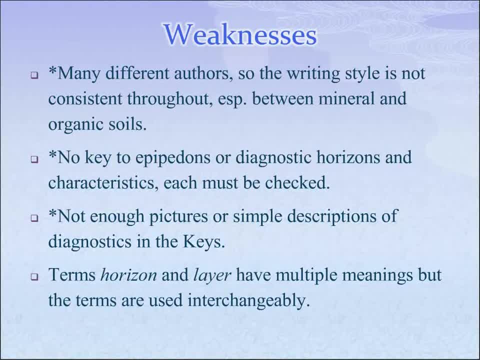 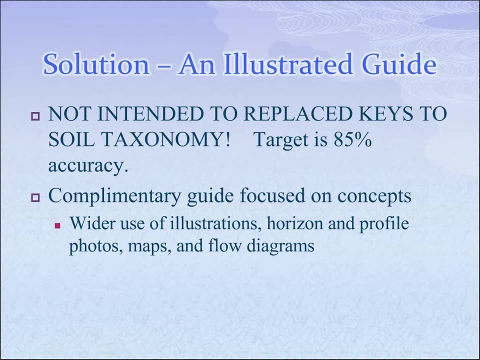 the inconsistencies of style there, no key to epipedons and diagnostic horizons and not enough pictures. you know that can be fixed or simplified through illustration. Yeah, And that's what this has been about, And that is what our solution is is the illustrated guide to soil taxonomy. 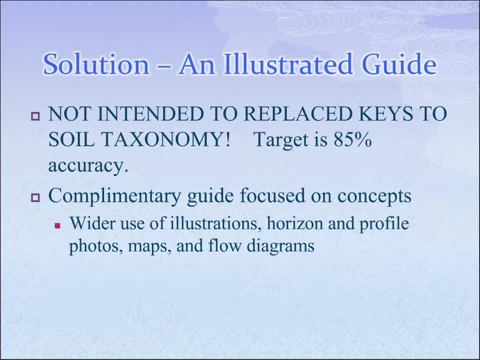 And one of the first things, you know, we want to say to those that are out there that are practicing soil scientists, professional with us, especially during the soil mapping program, and perhaps even those in research: this is not intended to replace the keys to soil taxonomy, nor soil taxonomy. 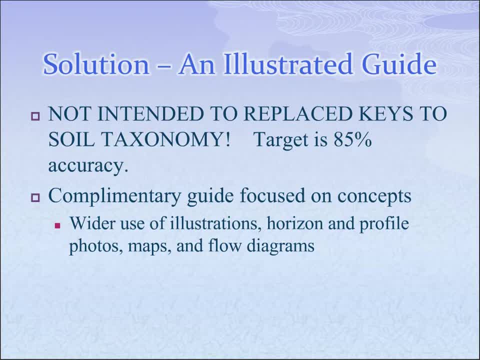 There are areas in which we know that if you follow the illustrated guide, it potentially can lead you to an error in classification. Typically. it's not Typically- though that would be in a very strict application of taxonomy- that it would lead you to such an error. 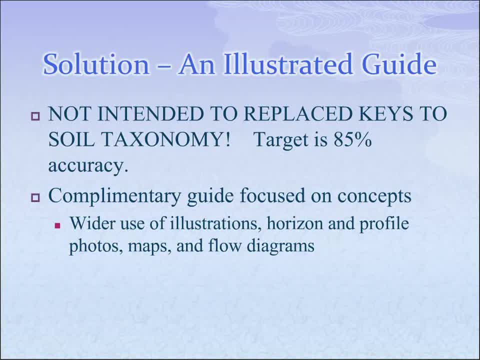 And in the case of student learning to use it, or someone wanting to know just about some general management of land based upon soil classification, the illustrated guide will probably serve your needs more than 85% of the time. I think it's interesting that some of our university professors that we work with 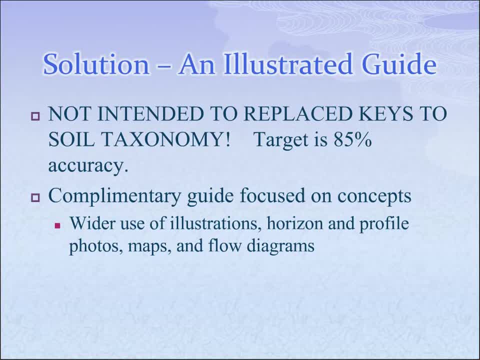 they believe that soil classification is important. They believe that soil classification is important. They believe truly that the accuracy of using the illustrated guide is much higher than 85%, easily over 90%. I don't think anybody's done any statistical analysis of that, you know. 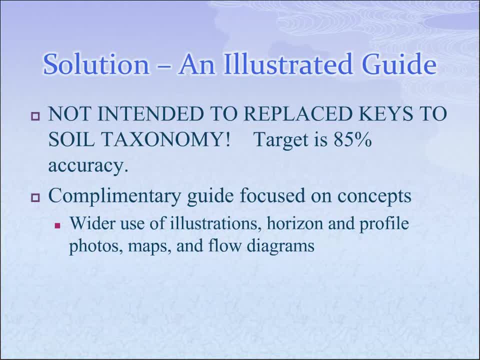 like classifying a thousand pedons and then seeing what they you know. did it match up to the correct classification? But the idea is you know most of the time it's going to get you to the right answer, But there are certain situations, particularly with sliding scale criteria. 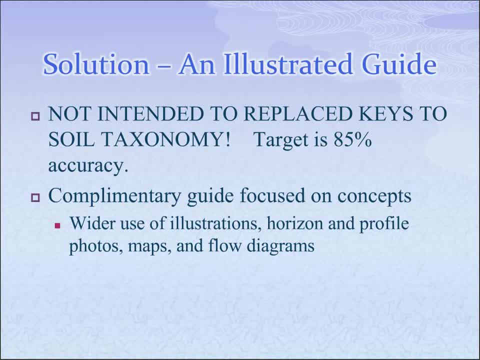 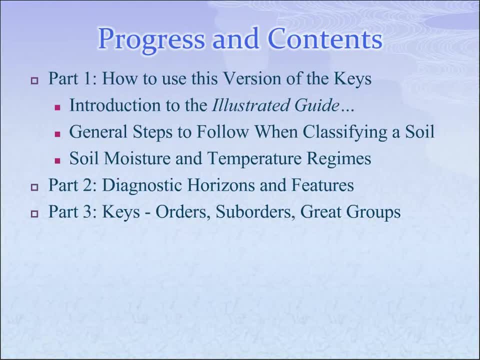 that you wouldn't come up with. you know that technically correct answer. Let's see the general contents we're working on. actually now a second, pretty much a second document, which is the illustrated guide. We had an earlier one that we had developed just in testing. 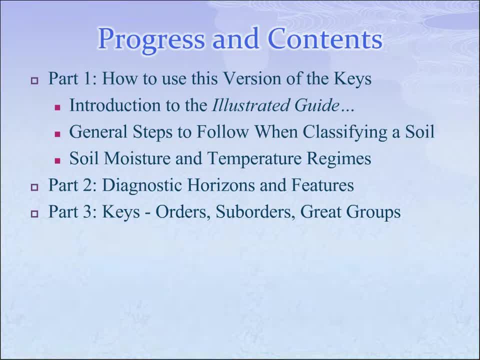 that was called the simplified guide, And we suddenly realized our simplified guide was completely full of pictures and illustrations and diagrams- And I don't know who it was- It was Craig or someone- come up and say: this thing's more like an illustrated guide. 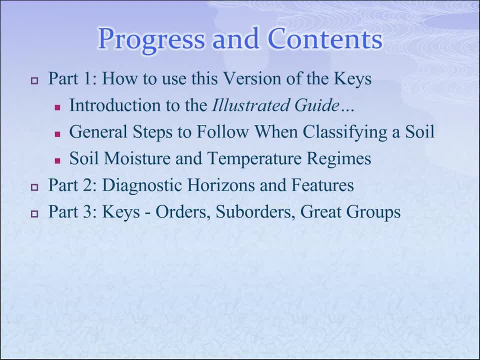 And that consequently, we did think that would probably be a better name for this document as an illustrated guide to soil taxonomy. It consists of basically three parts. One is the how to use this version of the keys. It tells you how to use this document. 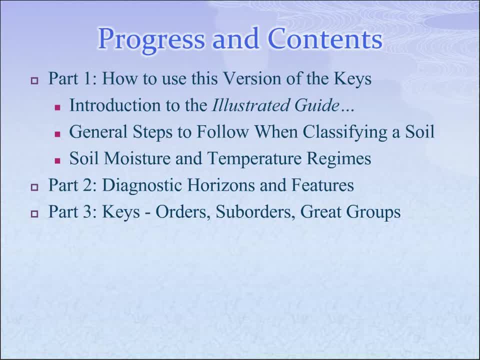 And it gives an illustrate introductions to the illustrated guide, some general steps to follow, You know, for a student, when they're just learning how to classify soil, how to go about what to look at and how to go about classifying it. 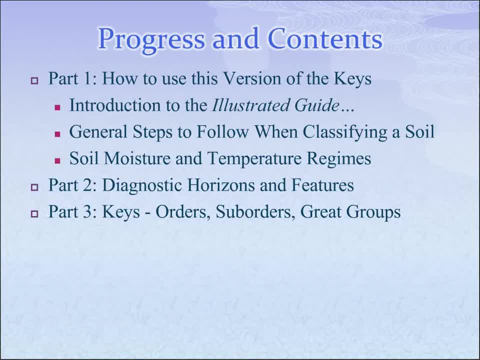 And then it has some information about soil and temperature moisture regimes. Part two is diagnostic horizons and features, And this is where a lot of the illustrations come in. If you haven't seen redoxomorphic features before you, could somebody could describe them to you. 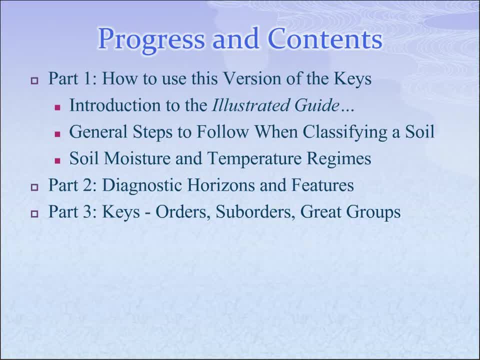 And after a little while you would probably figure out, okay, what kind of red areas and there's some kind of bleached out areas and such, But with a photo it's not. With a photo there, it's just immediate. 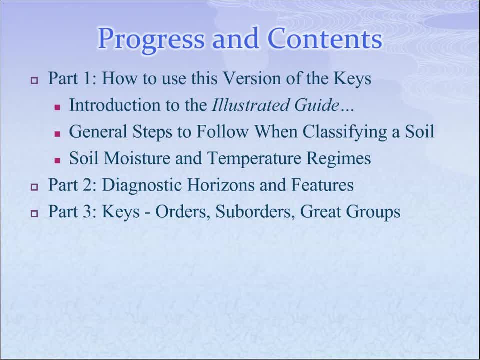 You know, your comprehension is immediate on what's being discussed, And so, within the diagnostic horizons and features, we have photos of almost all of those features within the soil that the students can use, The third and the main part, I guess, in terms of performing soil classification. 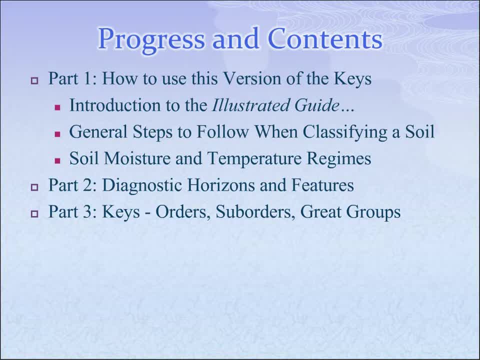 is the keys themselves, and it's keys to the orders, suborders and great groups. We only within the illustrated guide. it only takes you down through the great group in terms of classifying a soil And, of course, that is probably one of the main things that is taught. 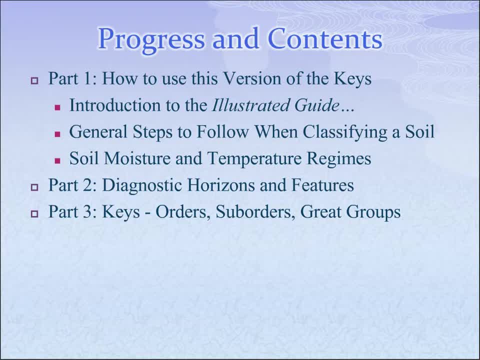 at the university level to beginning pathologists. We get into greater detail later on, after they understand the concepts of soil formation and the parameters that are looked at or that change as soils do form. And there's also a few other things included. There's a section on a few things. 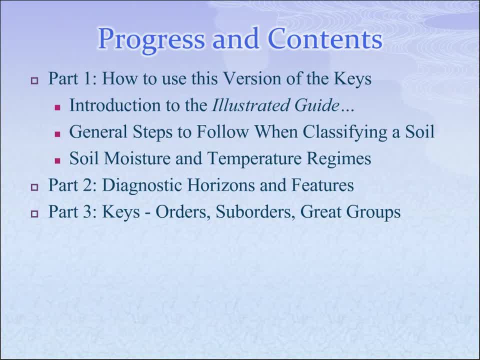 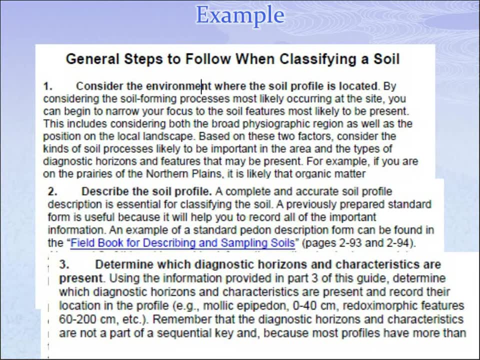 There's a section on a few things to know about classifying soils and some important sources of information you'll want to check out. We list some general steps to follow when you classify a soil in the illustrated guide And there's basically five steps. 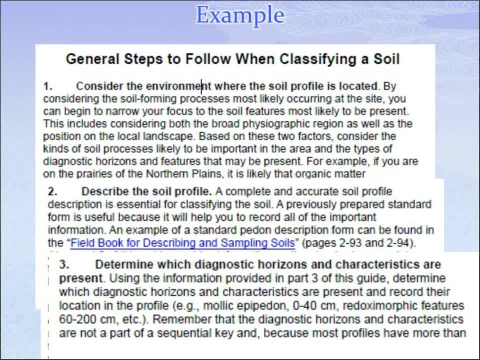 I've listed three of them here, And but you consider the environment where the soil profile is located, Then you describe the soil profile, Determine which diagnostic horizons and characteristics are present. The fourth step is identify the soil profile And then you describe the soil profile. 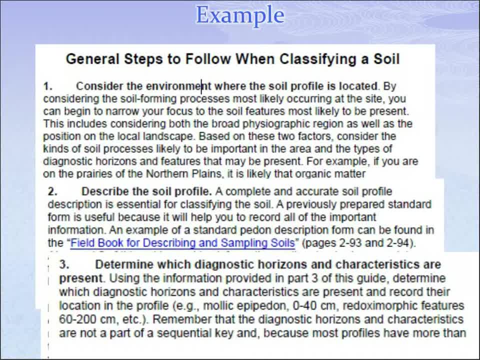 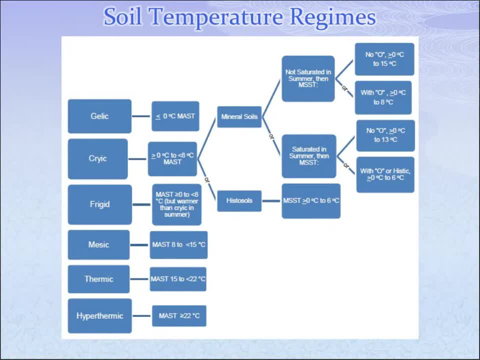 Then you describe the soil profile, Identify the soil moisture and temperature regimes, And then the fifth step is determine the classification. One of the things we've done here, you know, is put the- in this case, as you're looking at the screen- the soil temperature regimes into a flow chart. 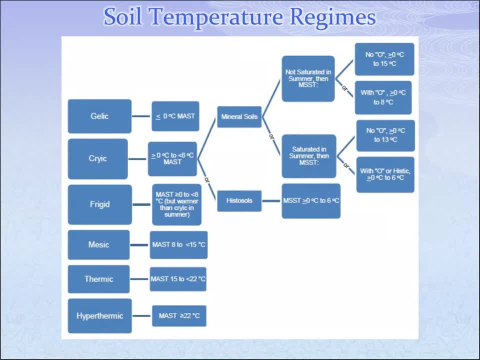 So you can see where you're at and you know how it moves. You know that if you're a gelic, you have a mean annual soil temperature less than zero degrees C In the case of cryic, if you are between zero and eight degrees C mean annual soil temperature. 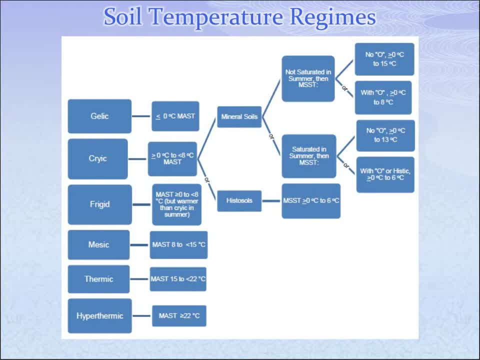 and you're in a mineral soil and it's not saturated in the summer, then your mean annual soil temperature, in the case of if you're not saturated, is zero to 15 degrees, or if it has an over horizon and if it doesn't have an over horizon. 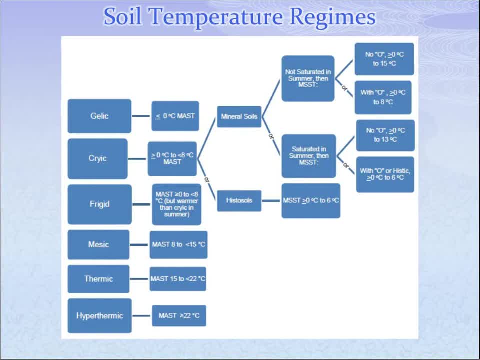 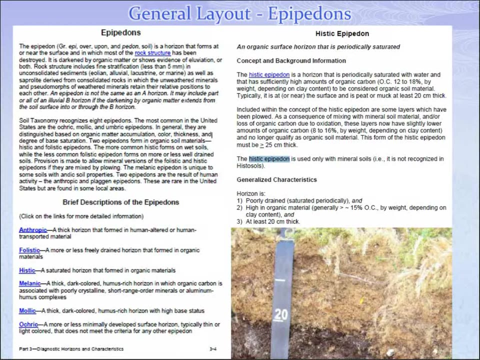 if it does have an over horizon, your mean annual soil temperature has to be zero to eight degrees, So kind of a way of walking you through this whole process of determining, in this case, temperature regimes. Here we've got an example of the layout that we used in the illustrated guide on this one dealing with epipedons. 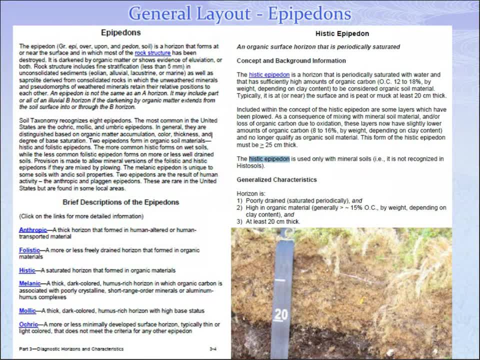 And so you can say we've got a, you know, sort of a simplified definition of the epipedon. Hyperlinks are used Really. the illustrated guide is made to use online, an online resource. Yeah, That's how a lot of our projects work. 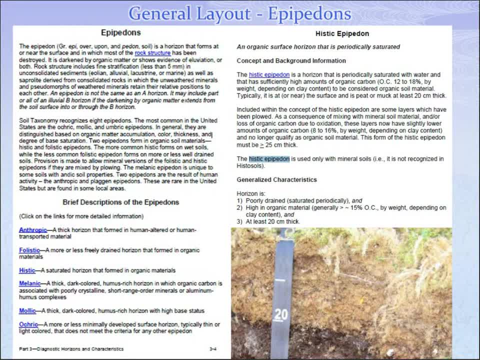 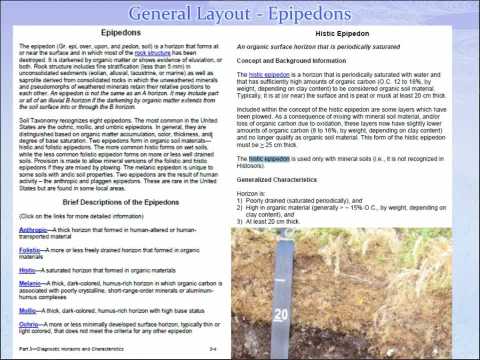 And then a picture that goes with it. So very visual. Yeah, One of the things we did too. when they're looking at it in the online version, it has bookmarks out to the left of the PDF, So that way you can jump very quickly to various sections of the document. 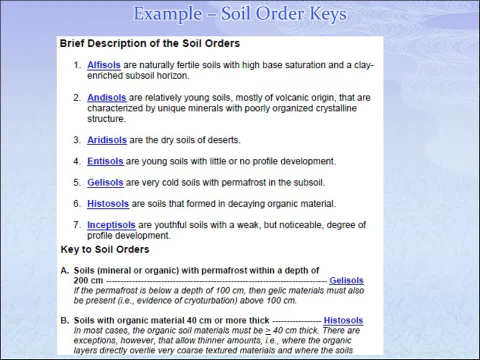 We give. within this we give a brief description of the soil orders and you see they are hyperlinked to a more, to a much longer description of the soil orders and it takes you through the entire system and it drops you down into the, into the keys. 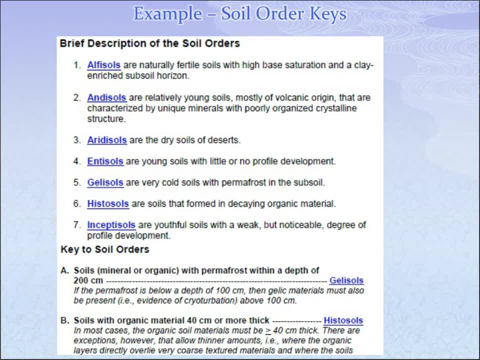 I'm not sure what else we want to say about that. It's basically this keyed out system where you simply walk your way down through the taxonomic classes. Along the way, though, much simpler definitions and explanations are given with regard to the various taxa group that you happen to land within. 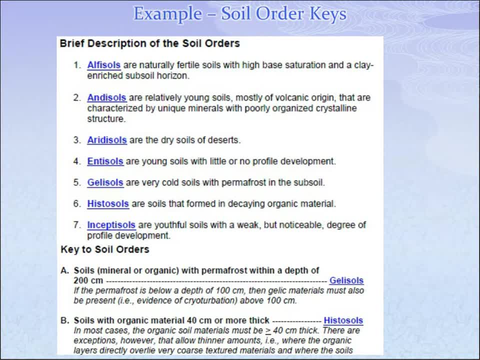 And a lot of these within. I think one of the big improvements that we've done with the illustrated guide is it gives descriptions of soils at the top of the taxonomic class. It gives you a little bit of an idea of what they are at that particular level. 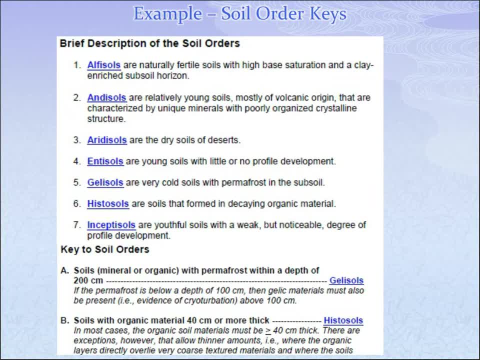 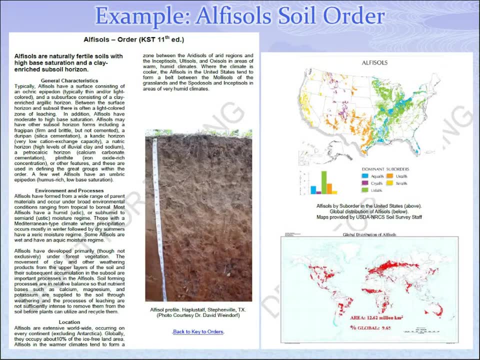 Making it a whole lot easier to comprehend the concept of what they are at that particular level. Shown now is an example of the of the alpha soils, and this is the general layout. This is again on one of the earlier editions that we had. 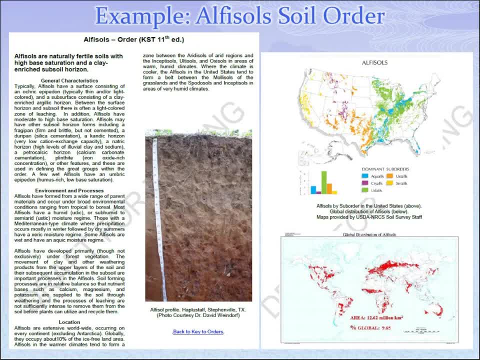 This was. this was a simplified guide edition. We now have the illustrated guide That is online, that you would be downloading and looking at, But this is how it- how it lays out, with the description of the alpha soils, the properties and qualities that and then, as well as it gives locations of the alpha soils. 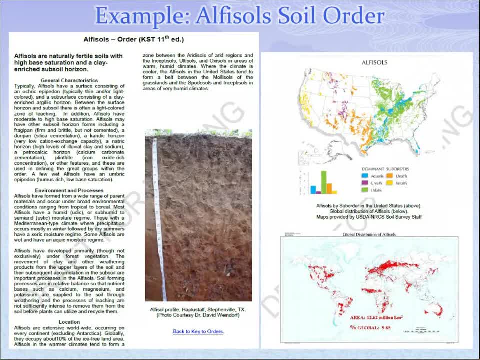 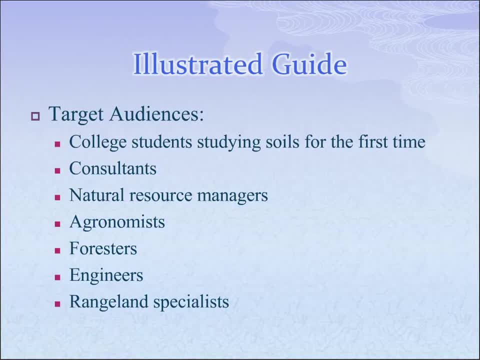 within the US and the and the suborders, as well as its the distribution of alpha soils throughout the world. So again, the target audience for the illustrated guide were basically those people that are new to soil taxonomy, So certainly college students studying soils for the first time, consultants. 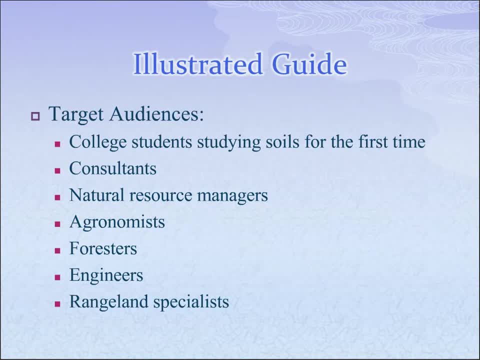 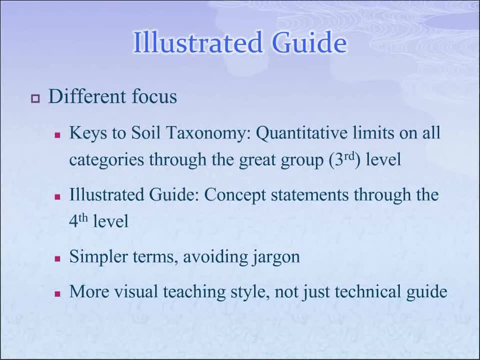 natural resource managers, agronomists, foresters, engineers, rangeland specialists. And there's a different focus on the illustrated guide. You know the keys to soil taxonomy. it has a lot of quantitative limits on all the categories through the great group level. 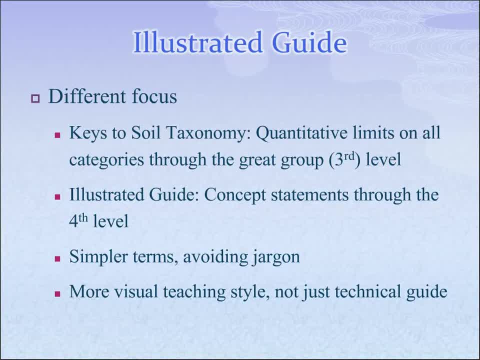 The illustrated guide got these concept statements through the fourth level and we've used simpler term terminology. we've avoided- tried to avoid- a lot of the jargon. You know it used to be the joke when I started as a soil scientist: you're going to read soil taxonomy. you have to be a lawyer. 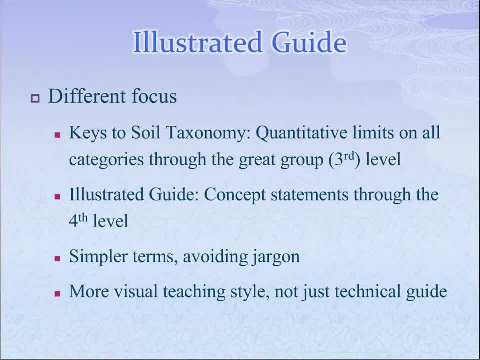 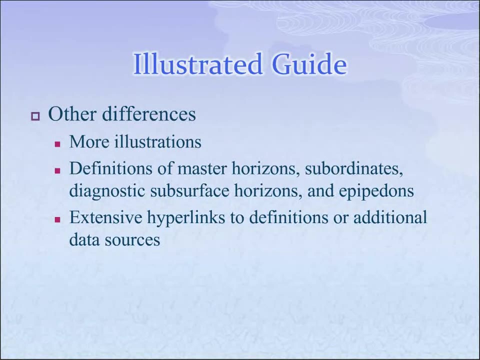 to understand what some of that language is. So hopefully we've tried to untangle some of that complex jargon that was used And, truthfully, it's a more visual teaching style. It's not just a technical guide. Yeah, Yeah, a number of the professors that we who worked with this, that has become 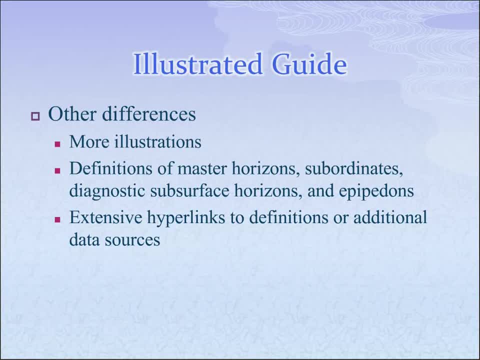 now this illustrated guide has become their textbook for their courses in soil taxonomy this year. Like I said, you know the illustrated guide. it has, you know, a lot of differences, a lot more illustrations, a lot more definitions and more clear. 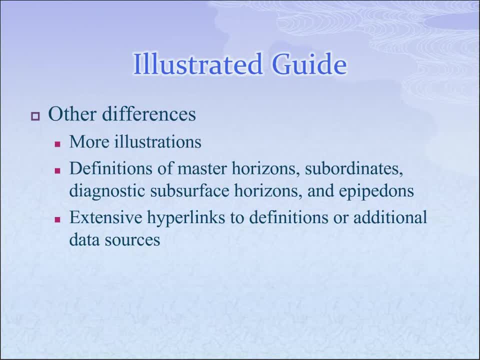 more simplified terminology used and the definitions of master horizons, subordinates, diagnostics, subsurface features, et cetera, And, one of the big things, the extensive use of hyperlinks. And not only will it take you someplace, 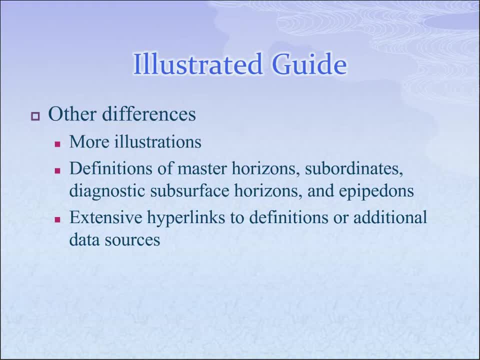 but with one click of the button you get to jump right back from where you came from, And so that's kind of a nice feature of this. So that way you don't have to lose your place when trying to figure out what a word means that perhaps you haven't seen before. 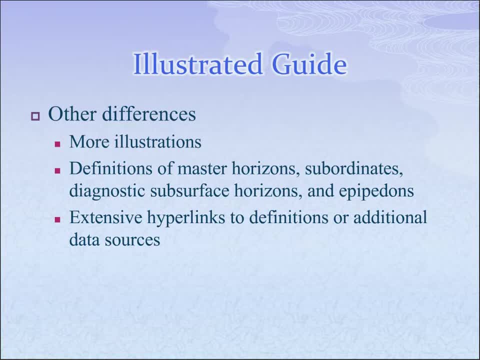 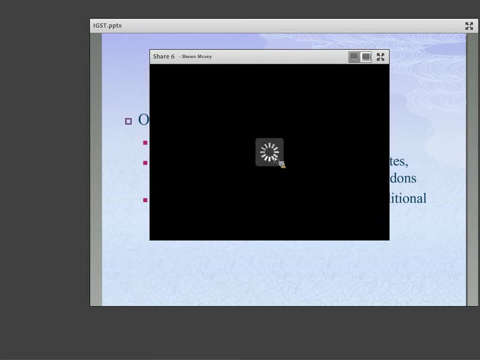 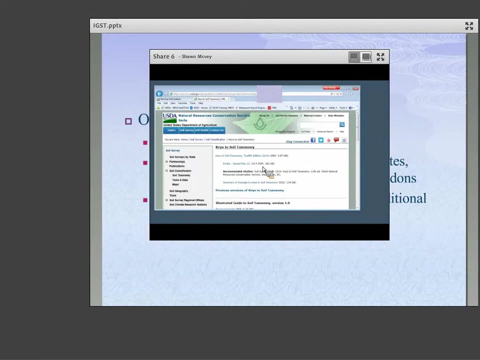 So that's almost the end of our presentation, but I'll just show you real quickly where you find this information. We'll get the screen shared in a second here. Here it comes. So, essentially, if you go to the what used to be called the soilsusdagov page, 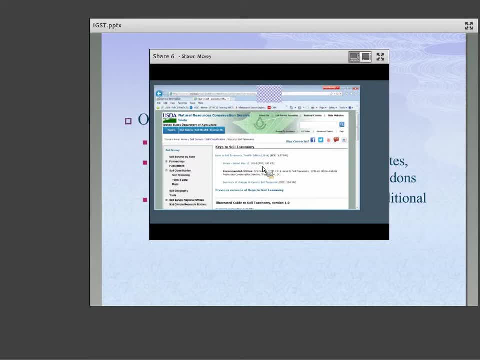 it's got a really long URL now, but if you search for soil classification and keys to soil taxonomy, you'll come up with this page, And this is where you get the keys to taxonomy 12th edition. of course, There's an errata sheet included. 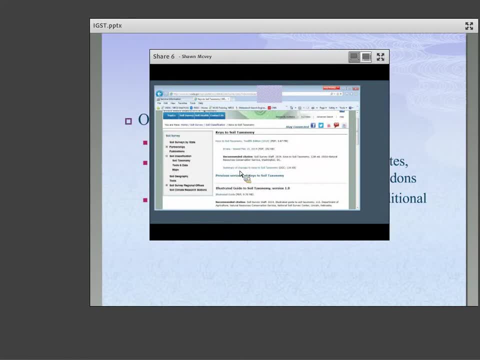 There's a recommended citation, summary of changes to the keys and then you've got previous versions of the keys And underneath that is the illustrated guide to soil taxonomy And it's a PDF. It's got the recommended citation, the illustrated guide description that we have online. 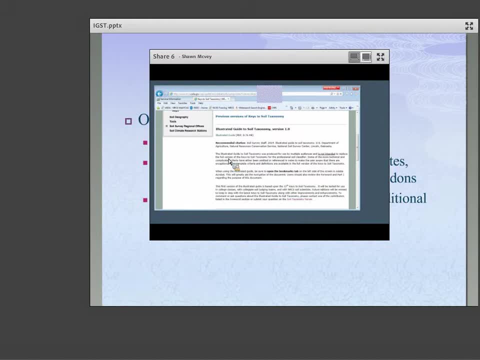 So it's really posted here for as much accessibility as anything. One of the questions that's already come through Ken is: is there going to be a hard copy provided of the illustrated guide? We have not. There's no plans for providing a hard copy. 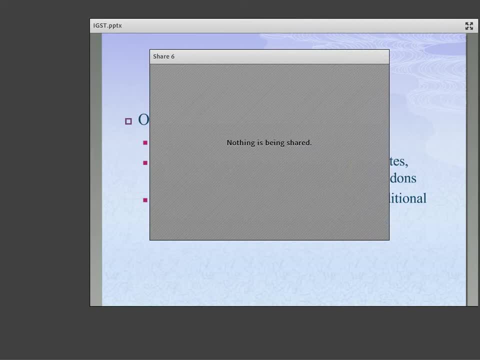 Because what we're actually looking at- we've already had suggestions for additional changes and improvements, And it's only been out since August- In a month, really, Yeah. So what we're actually looking at is the fact that this will probably be a very dynamic document, that we will continue. 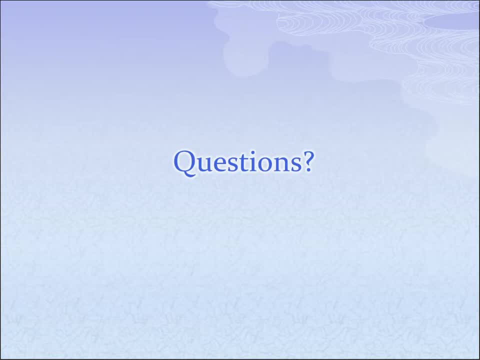 to make improvements throughout the year. We're thinking about maybe holding them solid by semester. That way a professor could have students latch on to one version. They could all work from that very same version. But I would, I would expect that we would be making changes and additions or improvements. 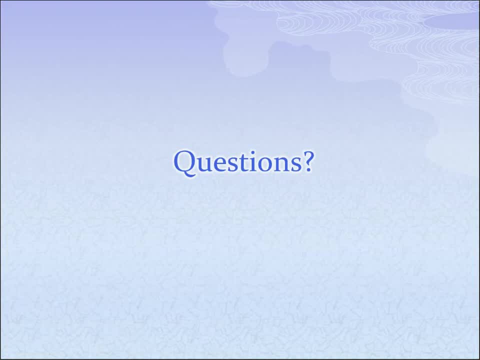 or whatever is recommended, on a semester-by-semester basis. One other thing about that: if you have any, if you've used the illustrated guide, the soil taxonomy, and you have comments or suggestions or you note errors that you think ought to be corrected, get ahold of us either on email, by telephone.